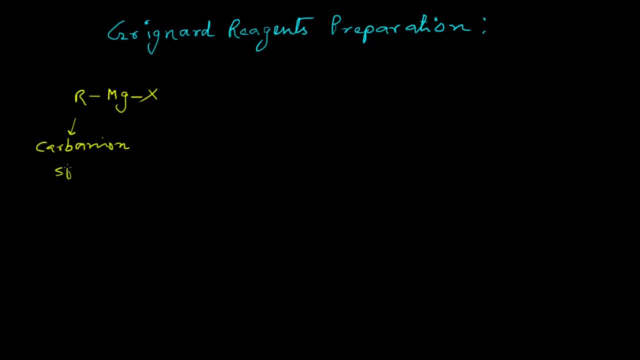 central carbon atom of this carb anion may be sp3 hybridized or sp2 hybridized, as well as sp hybridized, and this X stands for halogen atoms, which may be chlorine, bromine or iodine, but not fluorine. and if we consider the oxidation states, this magnesium is in plus two oxidation state. 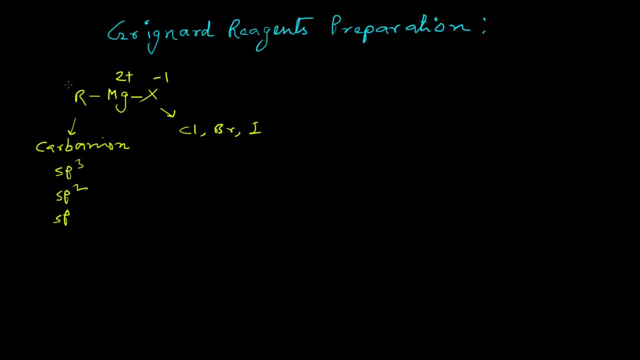 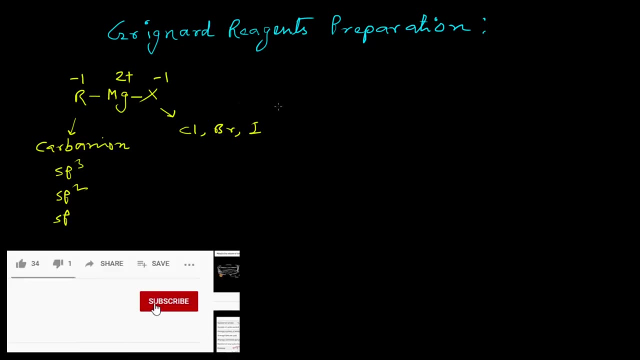 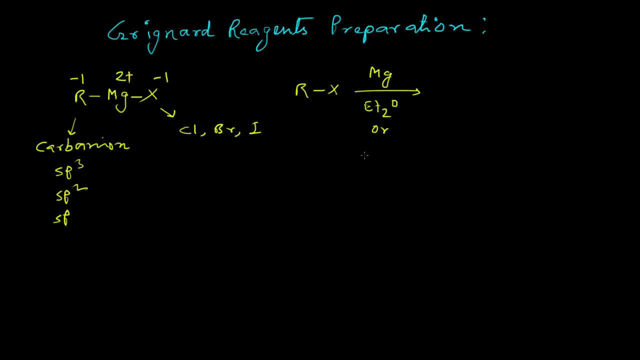 X is negatively charged and this R, being a carb anion, is also negatively charged. The basic synthetic procedure to prepare Grignard reagents are treatment of alkyl halides with metallic magnesium in ether solution, mainly diethyl ether or tetrahydrofuran THF, which has this structure right, and these ethers must be super dry. 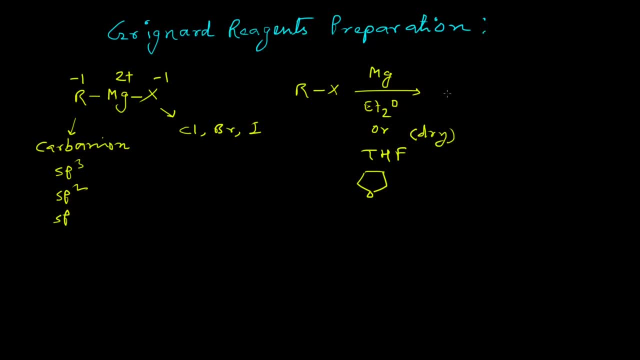 no trace amount of water should be there and after the reaction. the Grignard reagent solution will not break down in this structure and the nitr자�мос 적이 must be check After application. we will have to make the others necessary process like. 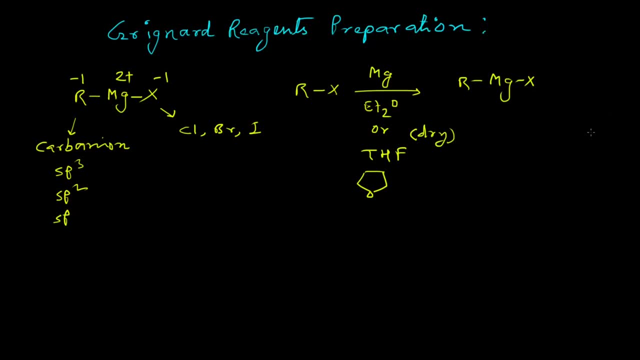 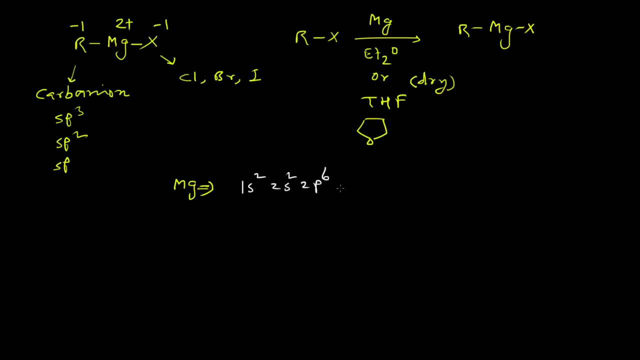 alcohol, lemon producot, heir throne and other relationships of whiplash techniques. Before we go into solution technology, let us consider. let us consider the electronic configuration of magnesium in order to understand how it reacts with this alkyl halide. the electronic configuration of magnesium is basically: 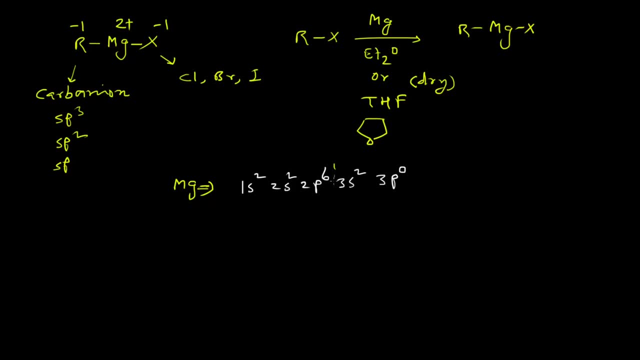 1H2,, 2H2,, 2P6,, 3H2 and the three Rabbi metals. relation to the Magnesium 3p orbital is vacant. its outer shell contains two electrons and that's why the valency of magnesium. 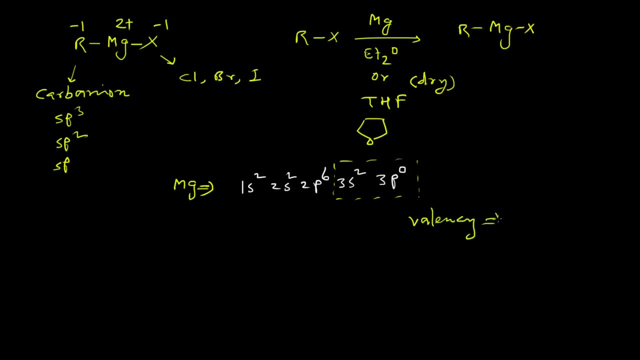 is two, which also suggests that in any magnesium salts or compounds the oxidation state, that is, the stable oxidation state of magnesium, should be always plus 2 right. so this also makes magnesium a two electron reducing agent. that is, if magnesium somehow is mixed with a oxidizing 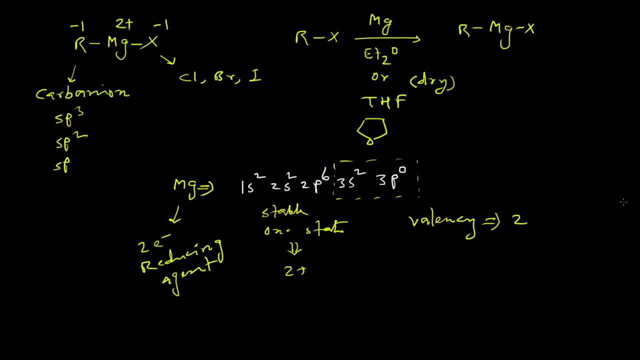 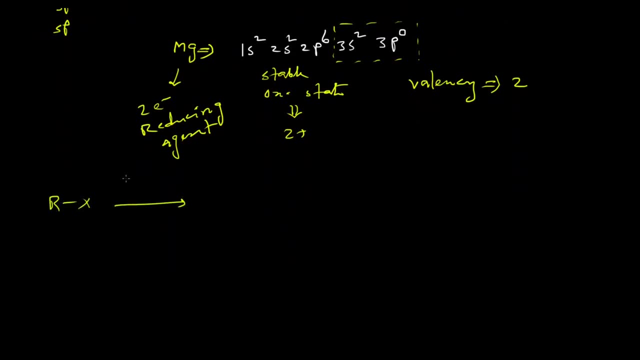 agent, then it will release two electrons to reduce that oxidant right. so now, if we consider the reaction between alkyl halide with metallic magnesium in ether, then obviously this magnesium will release its two electrons from this 3s orbital and it will undergo an insertion between this carbon halogen bond. 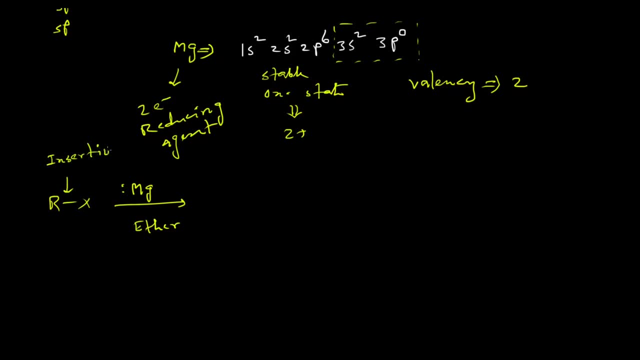 insertion. so basically the mechanism will look like this: magnesium will attack this halogen center by its electron pair and this rx bond will break. and as soon as this bond breaks, r minus will immediately get caught by this magnesium 2 plus which will form after the attack by this electron pair. right, 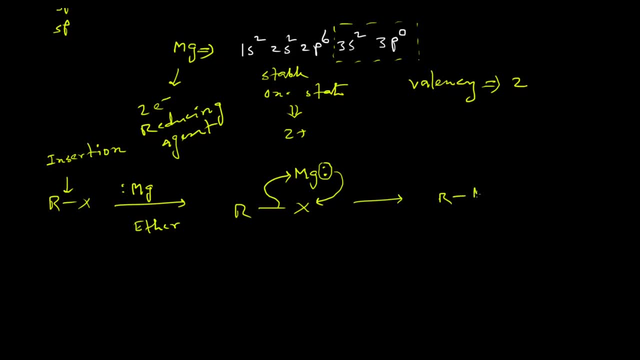 so this is the reaction between this carbon halogen bond and this 3s orbital. so this is the reaction between this carbon halogen bond and this rx bond, which will�. So here you can see that magnesium is giving its two electrons. that's why it will be converted into plus two oxidation state from zero oxidation state. x minus will be x will be in minus one oxidation state and this will form r, will form a carbanion, so it will also. 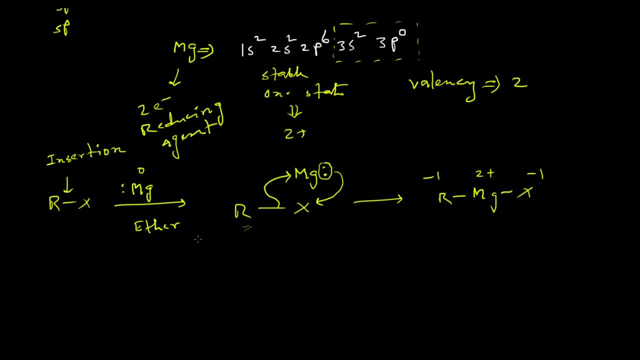 poses minus one oxidation state. Basically here, magnesium is almost indispensable to an oval ion. tenth and third Polus ion we can already see is being a very simple matter: o and so this magnet here, if you put x into r and v and then if you put r in the previousjat ionine, it will perform reaction through one single Имb arena from 0 information. 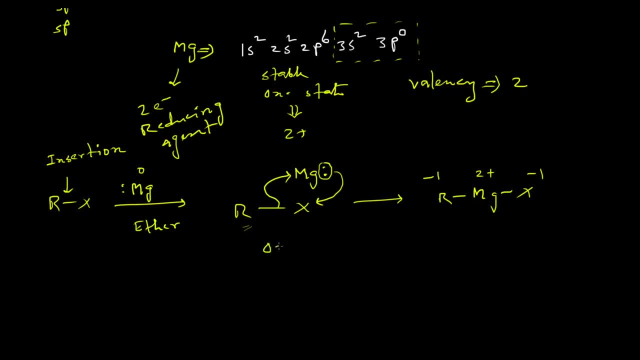 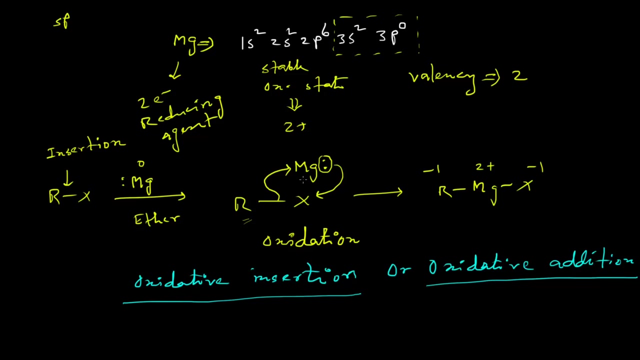 magnesium is undergoing a oxidation during this process. also, it is getting inserted between this Rx bond, and that's why this total process is called oxidative insertion or oxidative addition, right? either oxidative addition or oxidative insertion, both terms are equally applicable. so now you understand the mechanism of formation of this Grignard reagents, right? 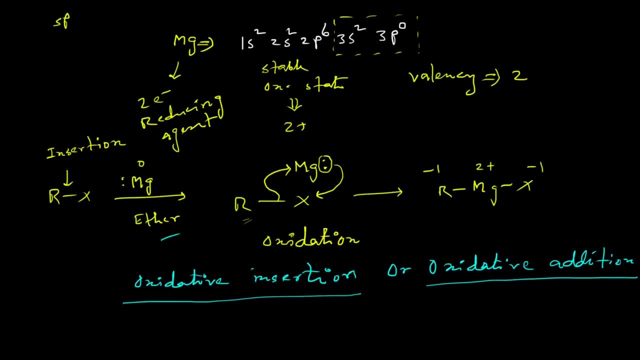 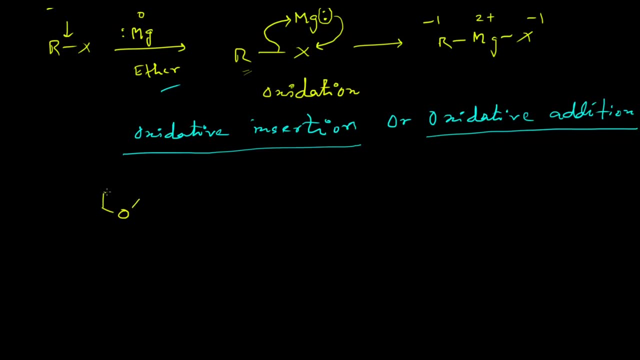 so what is the role of the solvent, this ether? if we consider THF or diethyl ether, both of them has a oxygen atom which possess two lone pairs, so it basically cold coordinates with this magnetic magnesium ion and thereby provides sufficient stabilization of this organometallic species. so this oxygen lone pair and this oxygen lone pair will undergo 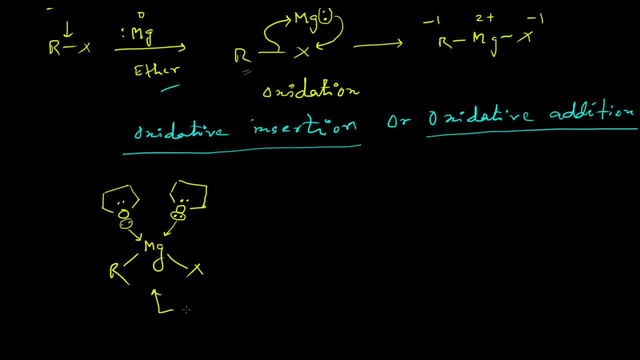 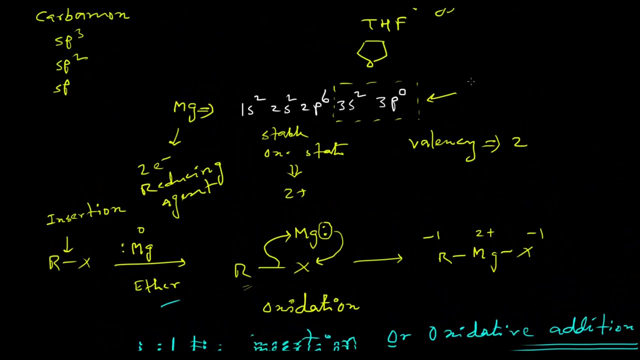 a interaction with this Lewis acidic center. it is Lewis acidic, So it's i. acidic nature can also be explained in terms of its electronic structure, since it has a vacant 3p orbital. thus it can accommodate extra electrons from any lewis base or any nucleophiles right. 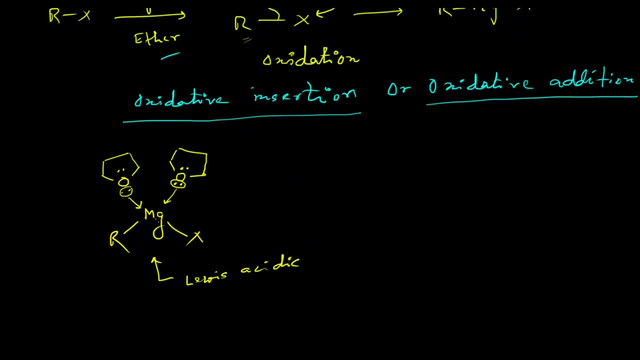 so here the two oxygen atoms are basically coordinating with this magnesium center, which is possible only because of the presence of vacant 3p orbital. so this type of interaction is stabilizing right. that's why ether solvents are generally used for the preparation or during the 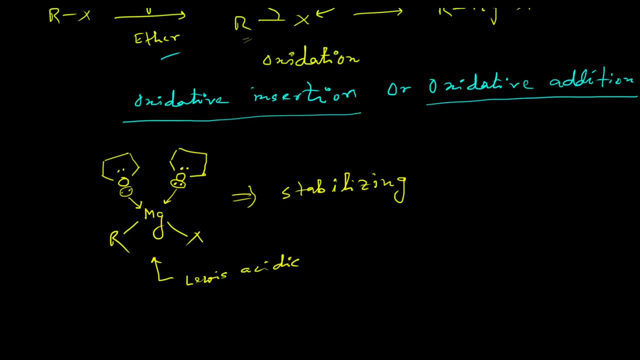 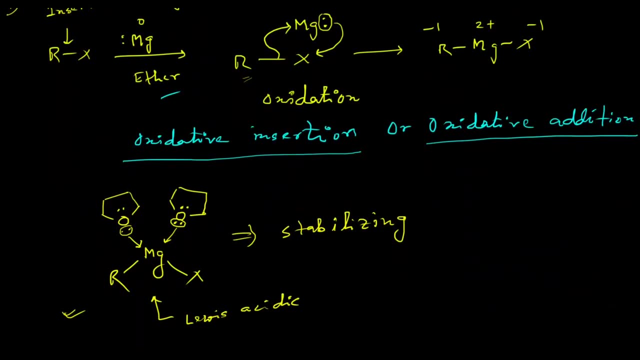 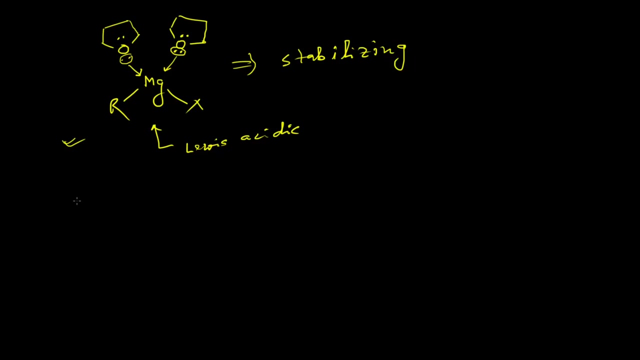 preparation of grignard reagents. so this is one type of preparation of grignard reagents, or where alkyl halides are reacted with metallic magnesium. let us consider some example and then i will go into other preparations. so if you simply treat two bromopropane, 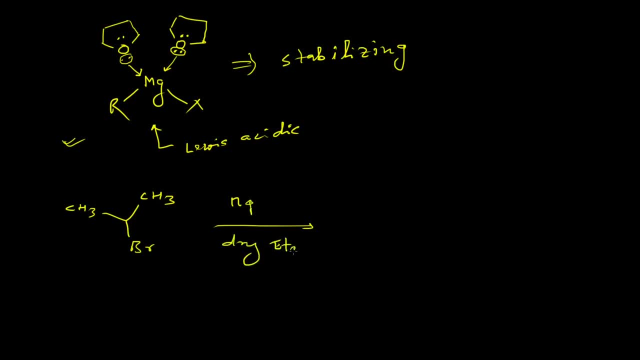 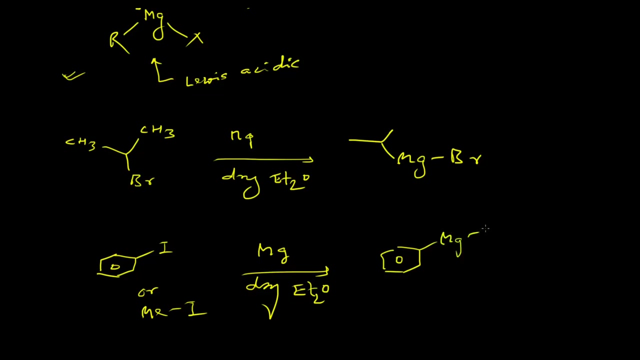 with magnesium in dry ether, you will get the corresponding grignard reagent right. another example is of iodo compounds. so if you treat this iodobenzene or methyl iodide with magnesium in dry ether, you will get this grignard reagent or this one. 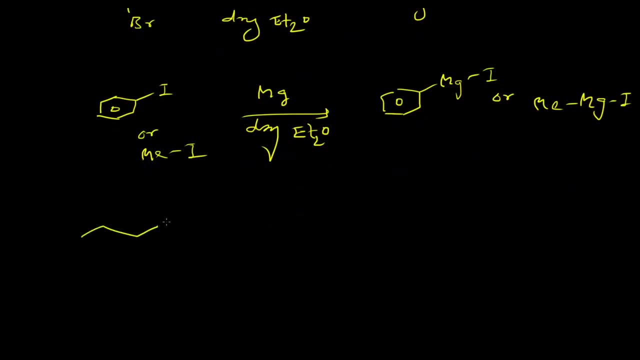 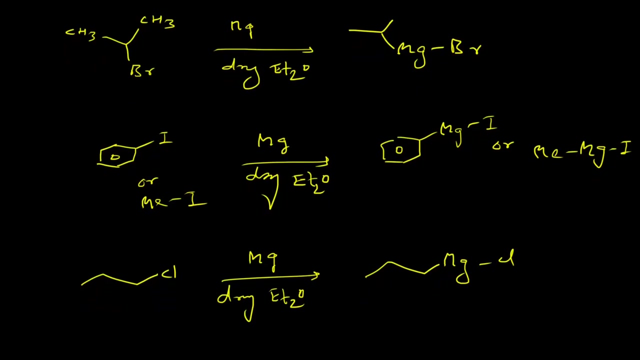 right половit urethane, and this example will be for alkyl chloride. in the same way, we will react it with magnesium in dry ether, and this will result in the formation of corresponding grignard reagent. so these are very straightforward procedures of synthesizing grignard reagents from 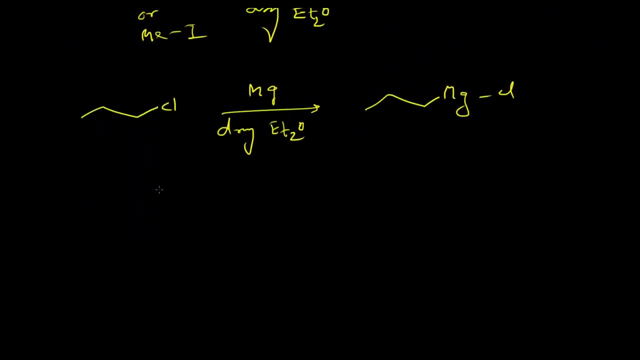 either alkyl bromide, iodide or chloride, so we can use, or we can use the right tool, in this case the. So let us consider the next possibilities If we react, let us say this Grignard reagent with an alkyne, which must be a terminal alkyne. 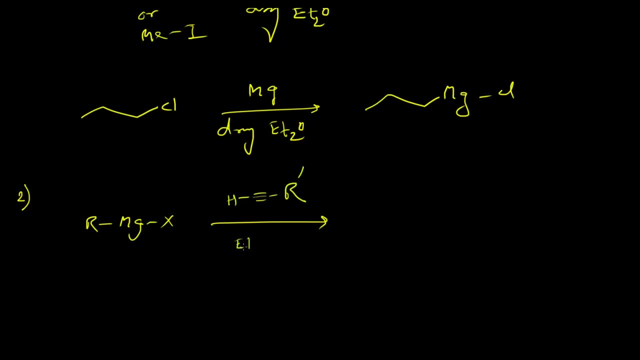 in ether. obviously, then, what will happen? this R minus will abstract this hydrogen atom from this alkyne, since this hydrogen will be acidic in nature, which is because it is attached with the sp hybridized carbon atom of this alkyne and due to the sp hybridization state of this. 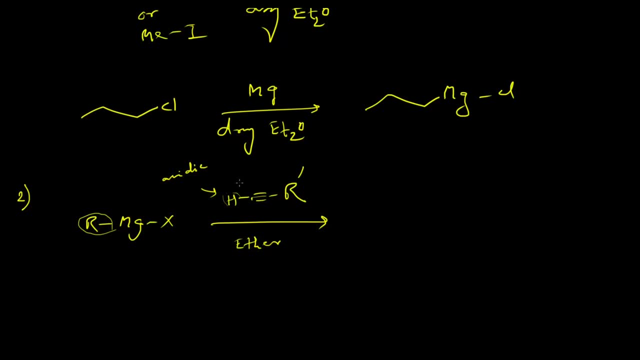 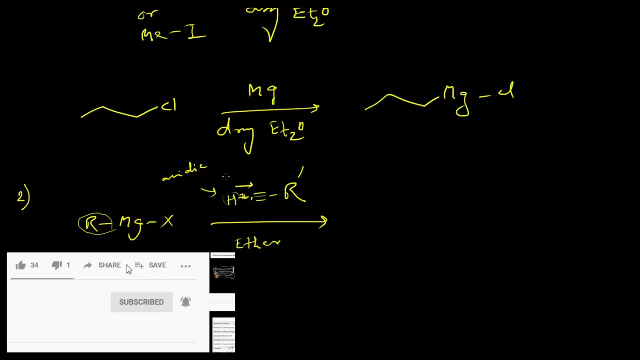 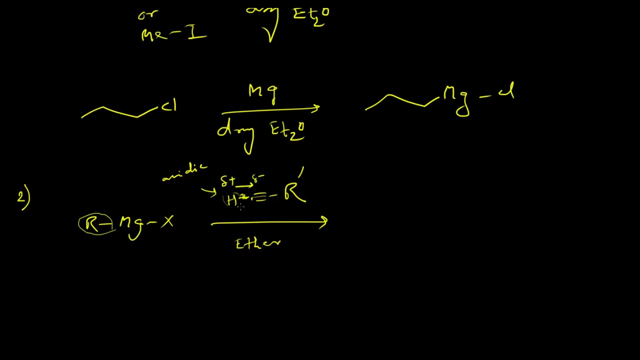 carbon atom, it will be of higher electronegativity and it will pull the sigma electrons of this carbon hydrogen bonds towards itself and thereby making this hydrogen partially positive charge Upon it and it will be partially negative charged. So that's why alkyne hydrogens are of acidic. 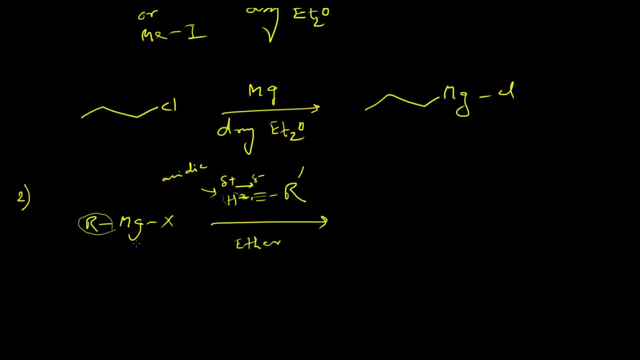 nature and due to this acidic nature, when Grignard reagents are reacted with terminal alkynes, immediately this R minus will act as a base and it will snatch this proton and it will produce the corresponding alkyne. and now, after snatching this hydrogen, 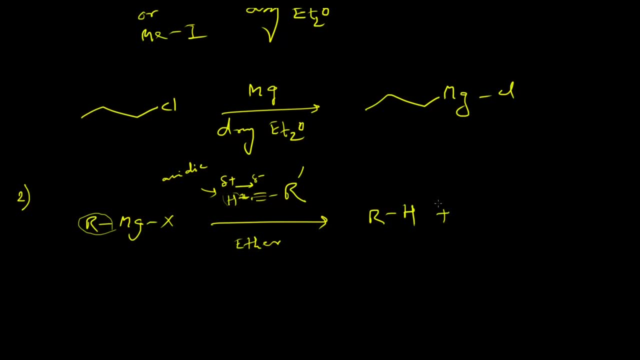 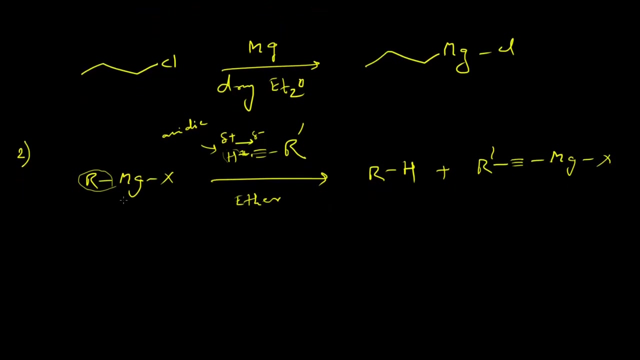 This newly formed carbon ion will combine with this magnesium center, so this will be our new Grignard reagent, right? so we are basically converting one Grignard reagent to another via this type of reaction, where it is basically reacted with an acidic hydrogen containing.